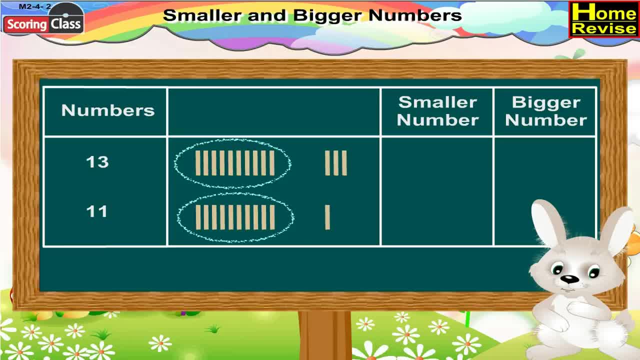 11. Now that you have created a group of 10 lines in both the numbers, let us find the remaining lines in number 13 and number 11.. In number 13,, three lines remain In number 11, one line remains. Well, three lines is bigger than one line, So 11 would be smaller. 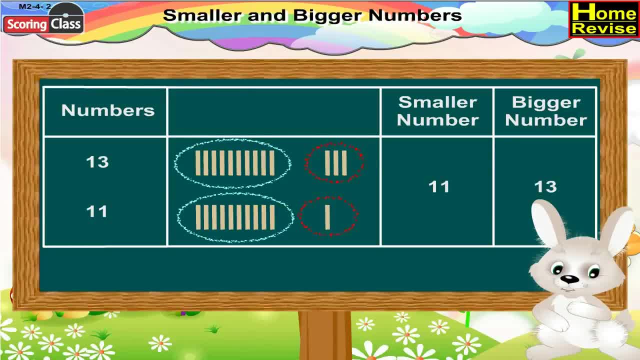 number and 13 would be bigger number. Now 16 comma 13.. Let us draw 16 lines for number 16 and 13 lines for number 13.. Now count 10 lines and encircle them for each 16 and 13.. Well, you have taken out the common group of 10 lines. 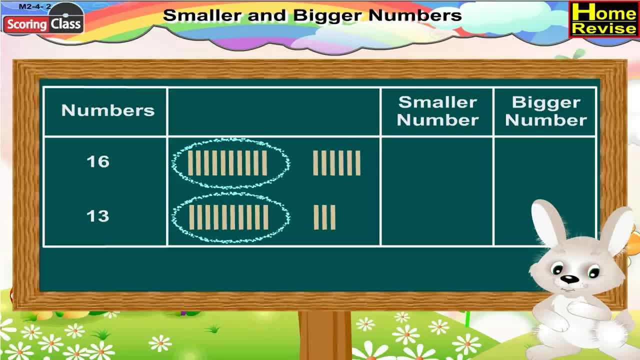 in each number In number 16,. six lines remain In number 13,. six lines remain In number 13,. 3 lines remain. Now 6 is bigger than 3, which means number 13 is a smaller number and number 16 is a bigger number. Now 10, comma 13.. Draw 10 lines for number 10 and 13 lines. 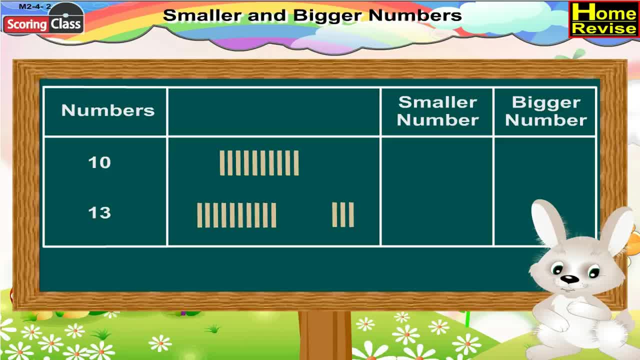 for number 13.. Now count 10 lines in each number and encircle them. You have created a group of 10. in each the numbers. Well, in number 10,, after encircling the 10 lines, no line remains In number 13,. after encircling the 10 lines, 3 lines remain, which means 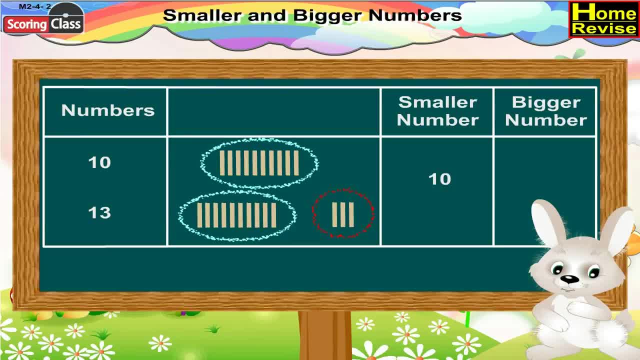 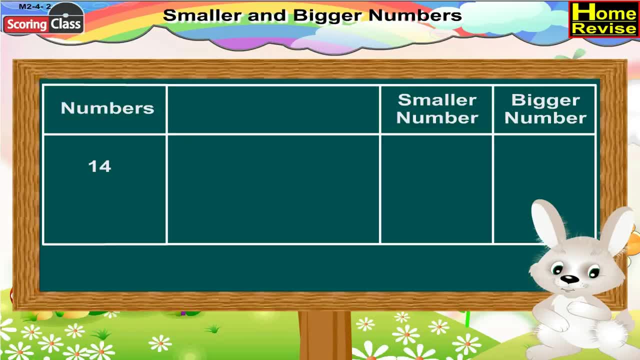 3. 14, comma 12. Now draw 14 lines for number 14 and 12 lines for number 12.. Now count 10 lines in each number and encircle them Now that you have created a group of 10 in each. 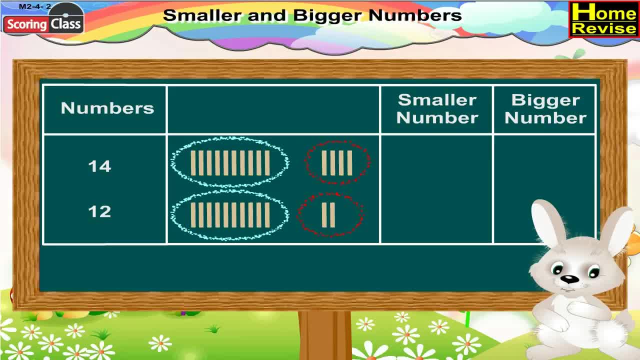 number. let us see how many lines remain In 14,. 4 lines remain In number 12, 2 lines remain. Now 14 is bigger than 12.. So number 12 is a smaller number and number 14 is a bigger. 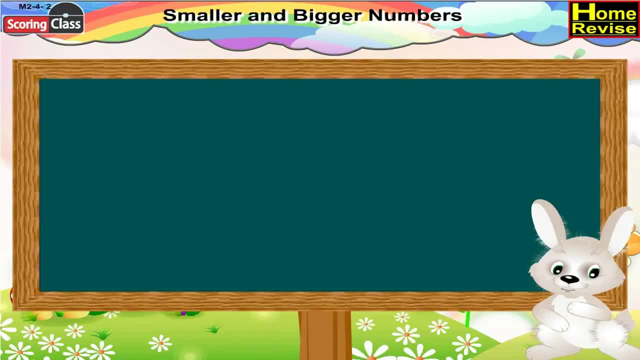 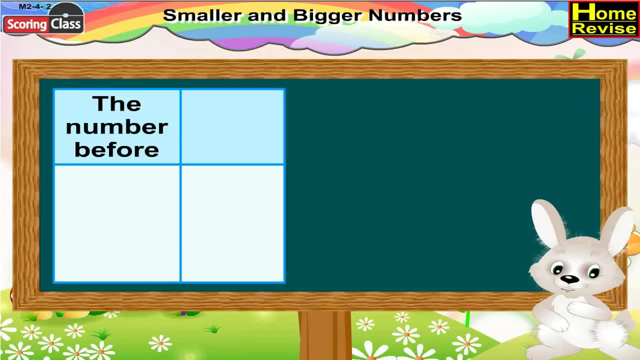 number Kids, I'll teach you a new concept. Let us find the number before. It's very simple. Let's start with 13.. Can you tell me the number which comes before 13? Start counting from 11.. 11,, 12,, 13.. So which number comes before 13?? You are right, It's 12.. 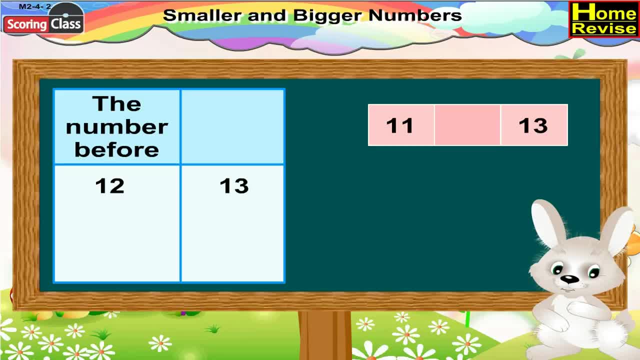 Similarly, let us find out the number which comes before 18.. Yes, it is 17.. Which number comes before 18? 1.. 1. number comes before 16?? Well, it is 15,, 16,, 17,, right, So 15 comes before 16.. And which? 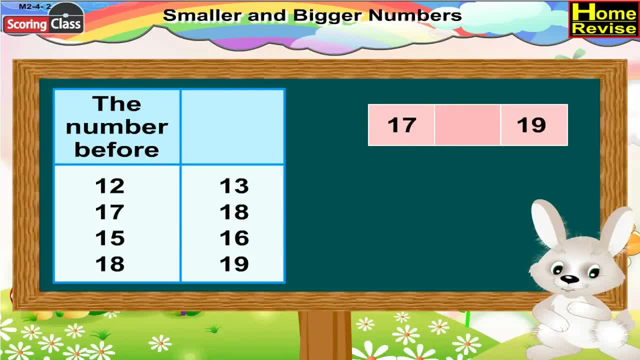 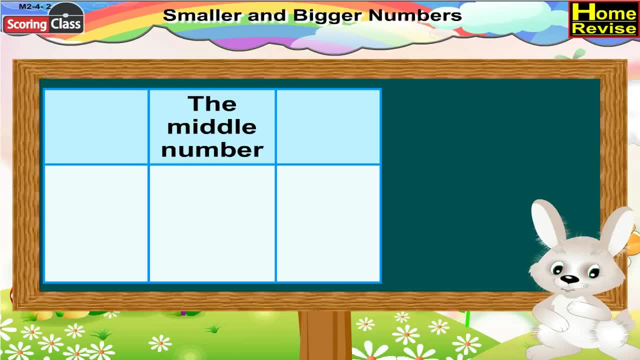 number comes before 19?? Yes, it is 18.. The middle number: Let us find out the middle number: 12-14.. Now, what comes between 12 and 14?? Let's start counting 12,, 13,, 14.. 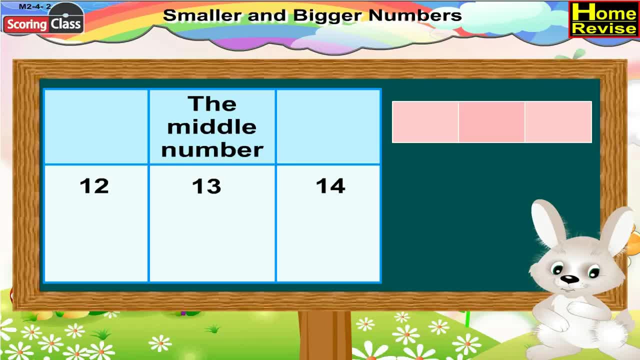 Yes, the number is 13.. Similarly, let us find out which number comes in the middle of 17 and 19.. Yes, it is 17,, 18, 19.. So the number is 18.. Now let us find the number which is in the middle of 15 and 17.. You are right, It is. 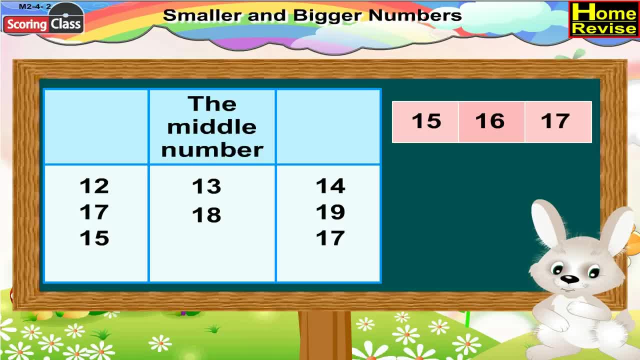 15,, 16 and 17.. So the number is 16.. Now 18-20.. Yes, it is 18, 19, 20.. So the number which comes in the middle of 15 and 17.. Yes, it is 18, 19, 20.. So the number which comes in the middle of 15 and 17.. Now 18-20.. Yes, it is 18,, 19,, 20.. So the number which comes in the middle of 15 and 17.. Now 18-20.. Yes, it is 18,, 19,, 20.. So the number which